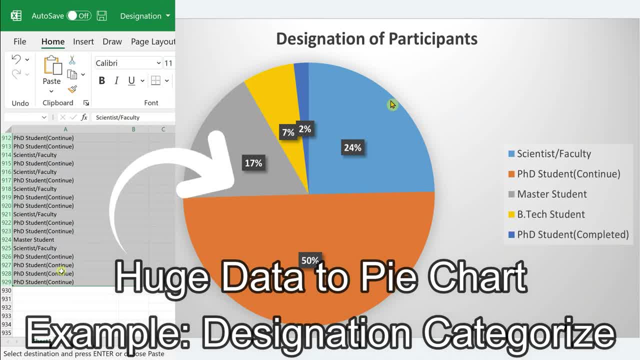 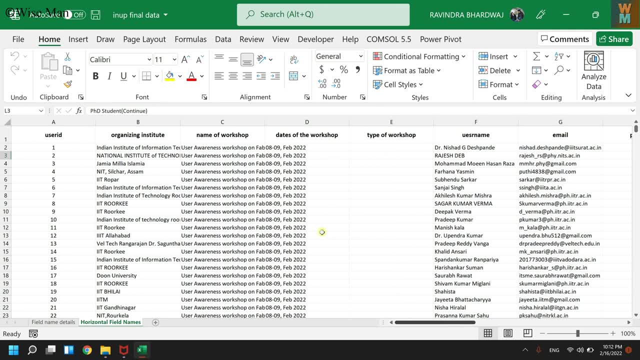 Hey guys, welcome to my channel, wise man, and today I will show you that: how can you take out data from Excel and how can you make a pie chart of that. so the data, what I means? that let's say you have a large number of data in Excel files, as you can see over here. 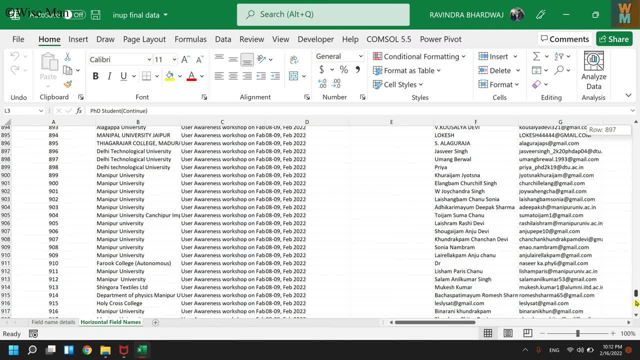 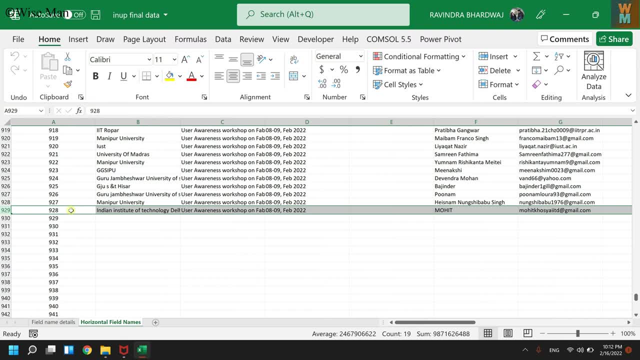 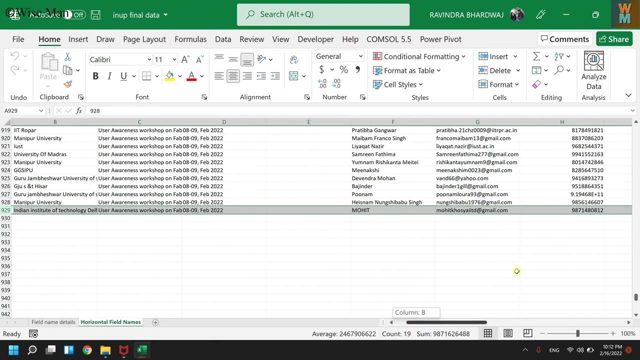 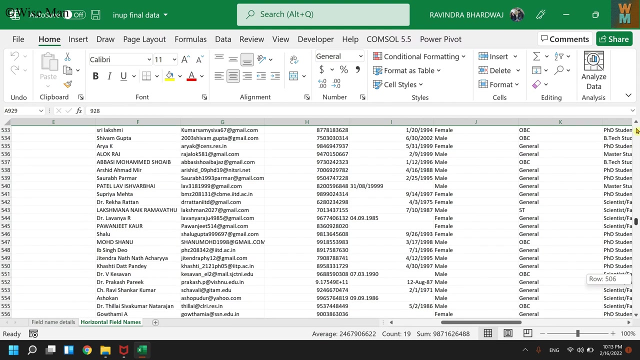 I have this file and I have so much data of about for around to 928 number of rows, right, so I have about, let's say, 928 members and I have data of 928 people's members and I want to make a pie chart. Let's say I want to make a pie chart of so in this data. let's say I want to discretize. 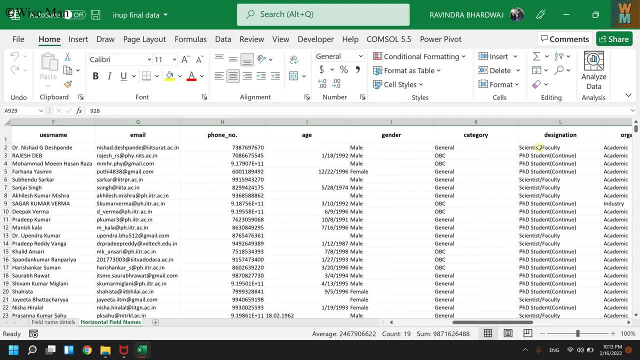 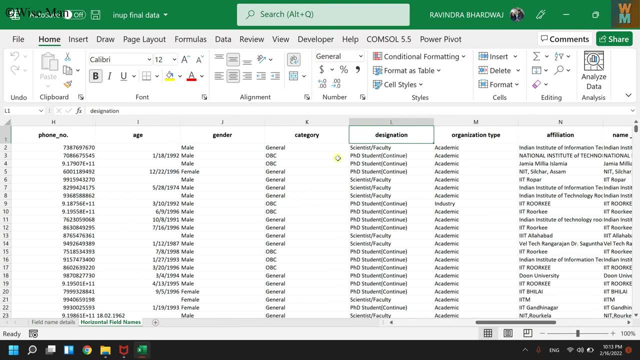 or I want to differentiate this 928 people's by designation, right? So let's say, I want to guess, I want to differentiate all these 928 people's in terms of their designation. so designations First of all. you need to see that, Okay. 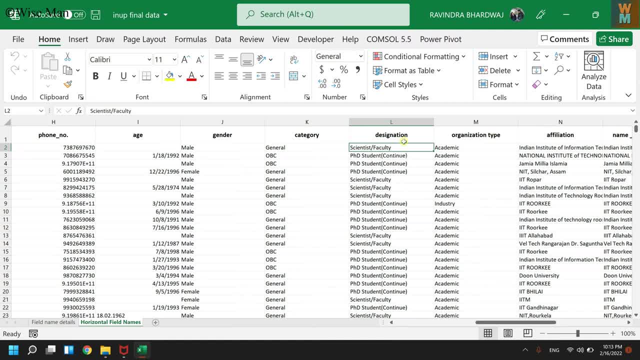 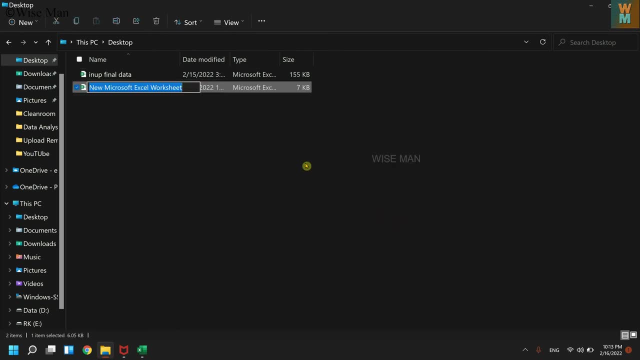 What are the designations you have in this column right? So, as you can see, it is very complicated. So what you will do, you will select this column and first of all you copy that and wherever you have saved this file, you can go create a new file of Excel and let's say it is designation. 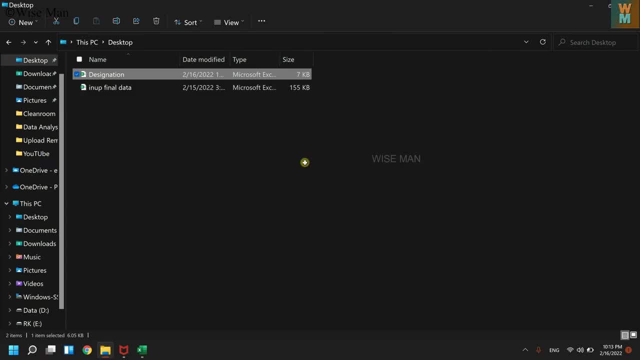 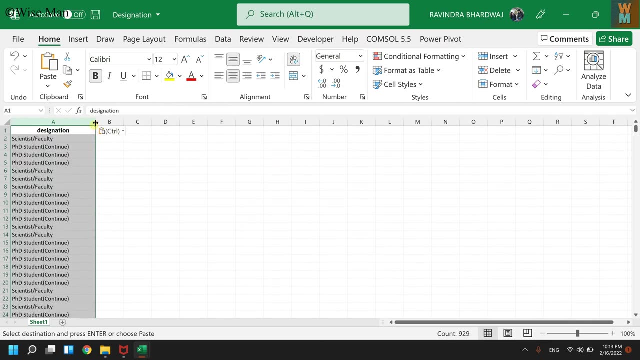 So just give a name of this file, designation, and I will open that file and I will just paste all this over here in the first column, Right. So I got all these things of what are the designations from row two and just hold control shift and press the down key. 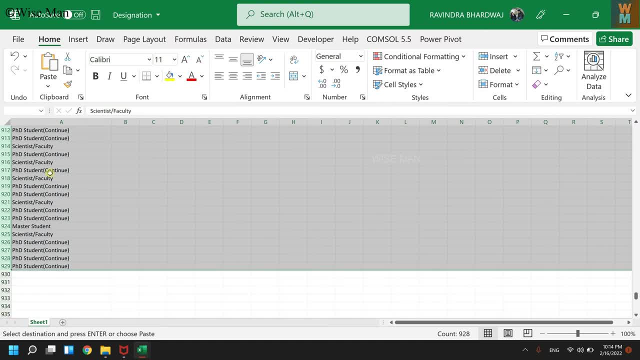 It will select all the number, all the values which have this data, right, It will not select below 930 because there is no data in that cell. so it will select all the cell which has the data till the end. Okay, So we got 929 and number of, let's say, people. 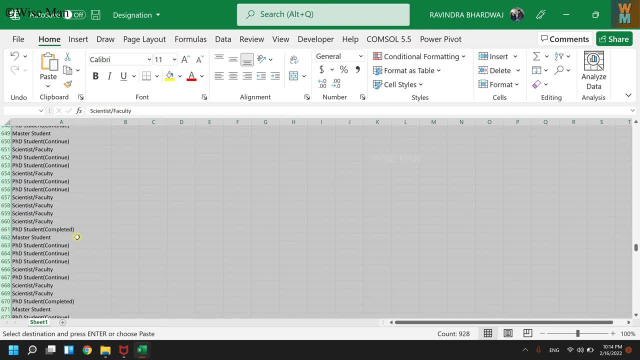 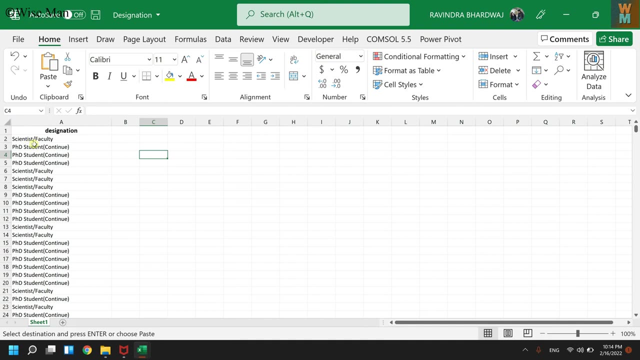 So now we have about, let's say, I think, five or six designations for all these people. So what I will do in order to quantify this right, I want to know, I want to get a number like, let's say, I want to find how I want to find. 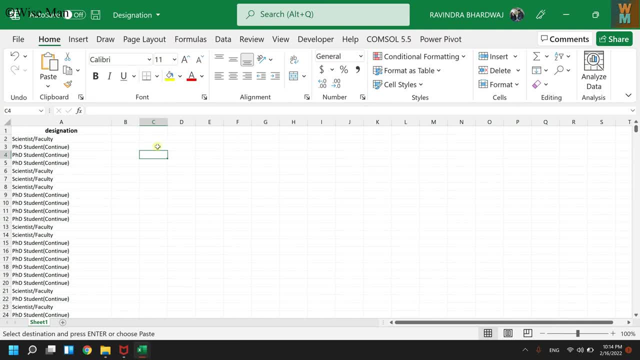 out that how many scientists are there, Right? So what I will do? Let's say I will make a column like I in this cell I will write scientist, or let's say faculty, right that cell. I will just write this one. and I need to find out from this. 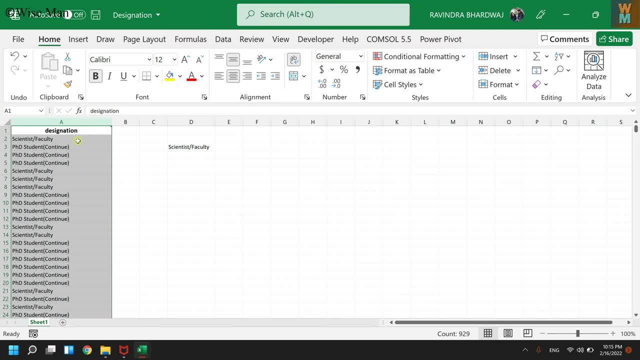 column, column a. how many peoples have this designation? So what I will do? I will write in front of this cell, from in front of this cell, Okay, I will write equal to and I will write count if right, so count if function, it counts the. 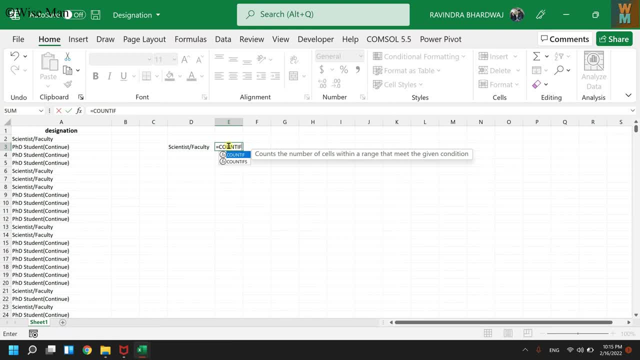 number of cells within a range. that means the given condition. So I will provide a condition and it will find out how many peoples have this designation Now I. then I need to define the range- So range is from this cell- and then hold the control shift and press the down key. 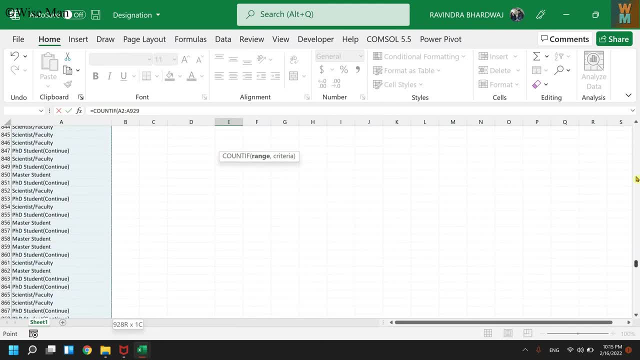 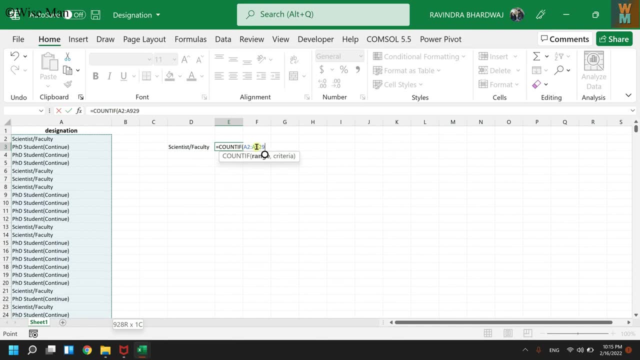 Right, So it will select up to the end And then we'll go up so it automatically selected A2 is to A929. that means it has selected cell A2 to A929 and then press the comma key, write the criteria. So criteria is: I want to find the cells containing this phrase or, let's say, this word. 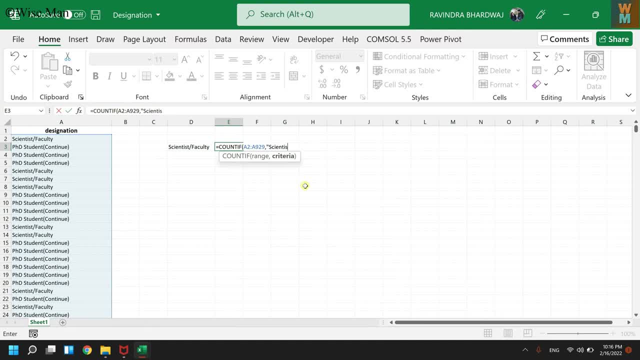 So the word is S-I-E-N-T-I-S-T, less And one more thing. Okay, One more thing. You can write in short Right: F-A-C-U-L-T-Y, So you don't need to worry about the captions or, let's say, the full capital words. 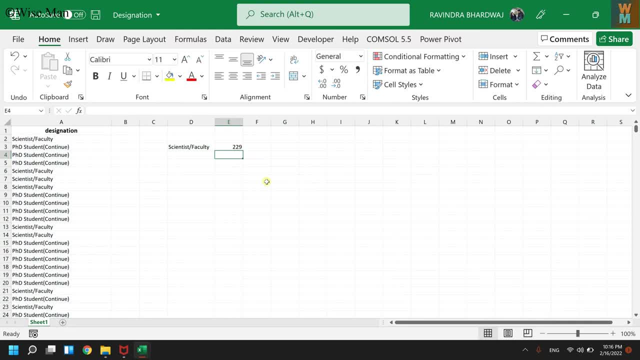 Then press and then close the bracket. press enter, It will find Okay. So it will count that there are two to nine peoples having this designation Right now. I want this also, So I will just copy paste all these designations. So PSD continue. 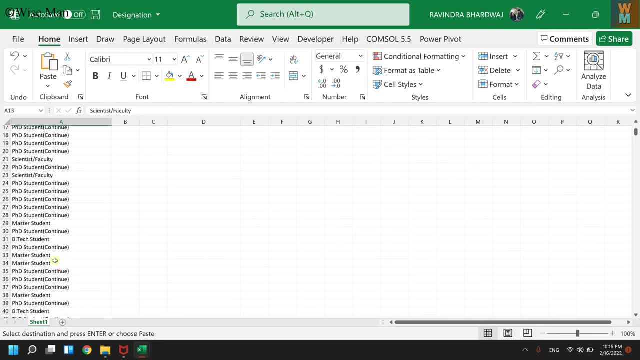 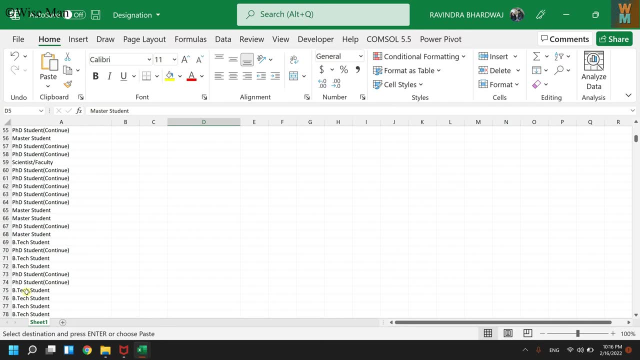 And then we have Master students- control C, control V, And then we have P-TECH students- control C and control V- Any other, Okay, So we have this also PSD completed: control C and control V. So again what I will do. 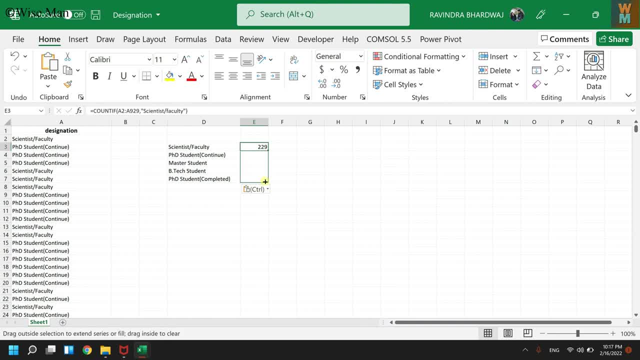 I will just, I will just, I will just Scroll this so that it will automatically take some default function. I will just change now So it is saying A3, I want from A2.. Then over here the criteria is: So for this cell, the criteria is PhD student. 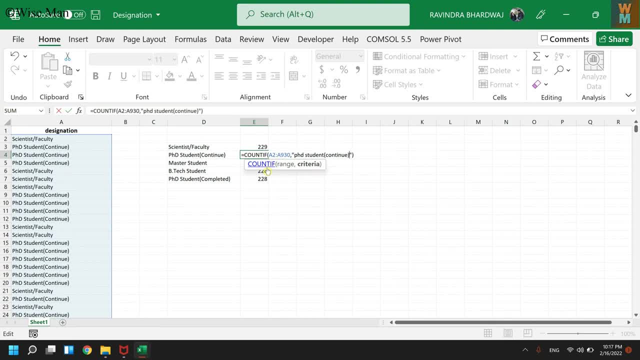 And then in bracket is continue Okay. and then press enter so it defines 463 students and over here it's again a2, and then it's master students, so write m-a-s-t-e-r-s-t-u-t-e, it enter 56 and then again it's from a1, sorry, a2. 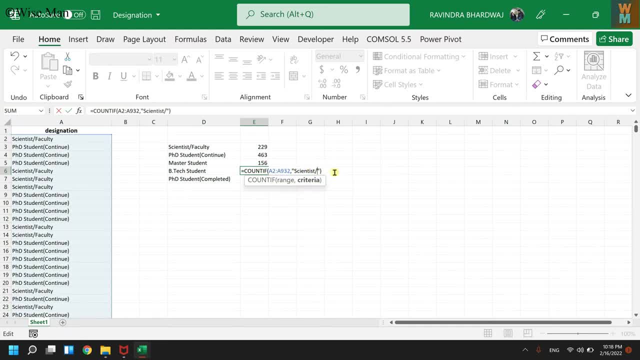 and then over here it's b tech student, so it's b dot, e-e-c-h, b-e-n-t, and then we have the adjustment completed. so again, a2, that you have to change the range you have to change, but be sure you provide the range which is required from where you need to find out this. 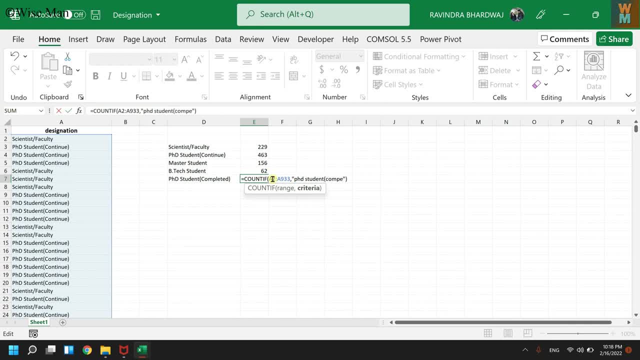 data. so it is complete. i get closed enter and now i just need to be sure that the summation of this is the summation of this, right? so let's say we have total which is equal to sum. i will write sum from this to this and it will give me 928, which is right because 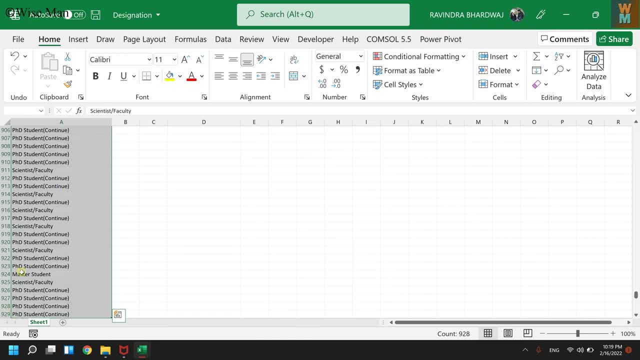 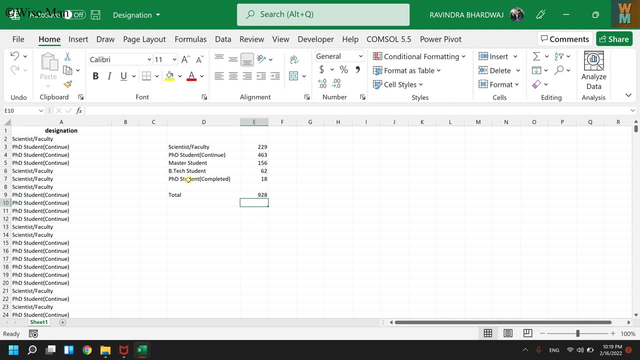 if i select this, i have 929. so i will select the top field, top cell, because it is giving me designation. so it is 928 students, 928, let's say members. so it's fine for me. there are five, uh, five, designations. now you have um justify, you have quantized, you have quantified the, the number. 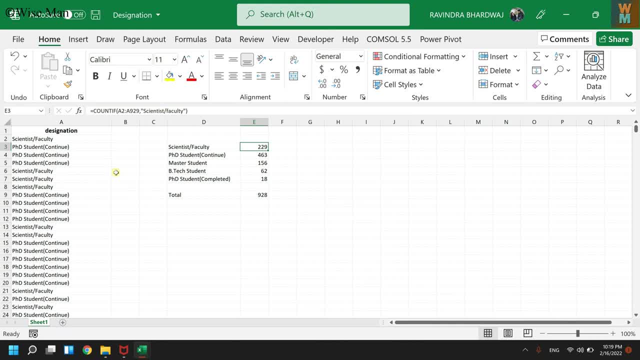 of the. you have quantified the numbers right now. we need to make a pie chart, right, so i have a pie chart. you just need numbers and corresponding uh phrases or things. right, rest right. because the numbers are corresponding to something, so that thing is uh designation over here. so we need a phrase and corresponding number for making a pie chart. so what you will. 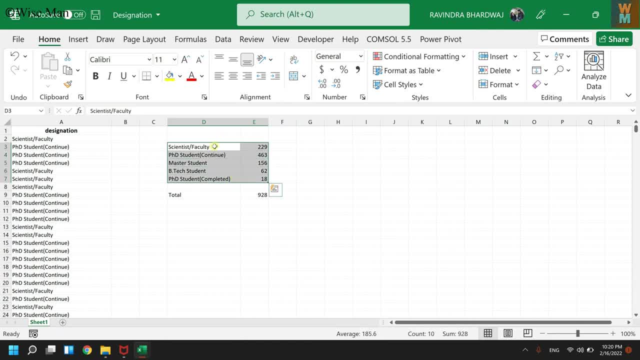 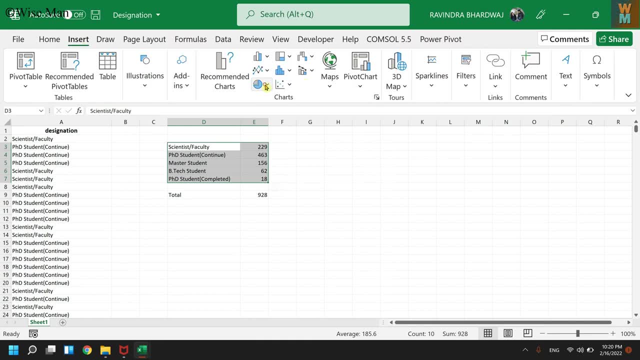 do? you will select all this, uh, all these cells which contains the designation and the values of the pie chart, and then you can see, you can find this, uh, if you are not seeing well on the back side what you can do, uh, you can go to recommended chart and then you can find. 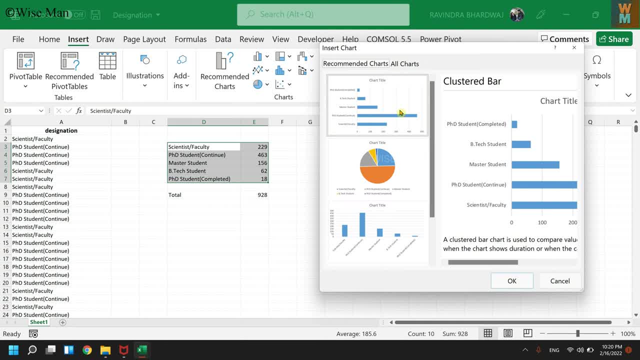 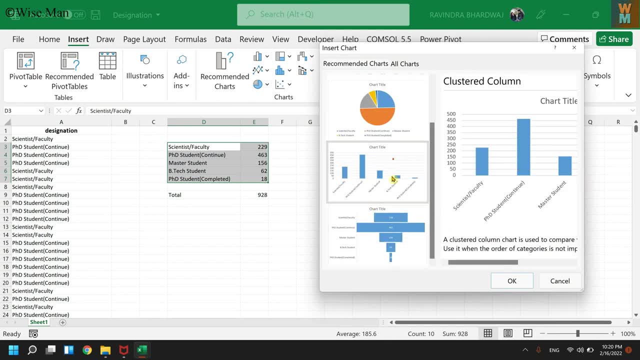 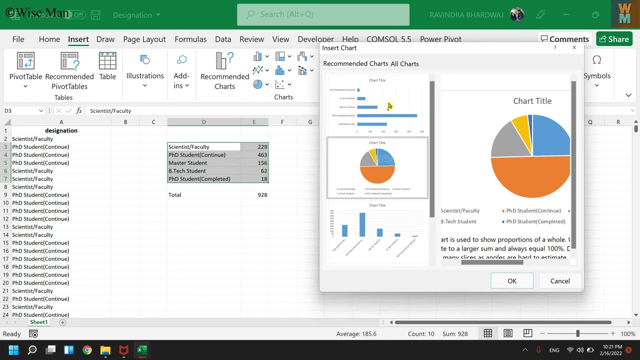 you can see that excel will recommend it use some charts. so it has this cluster bar pie chart. it will recommending. it is recommending a cluster column and chart and the funnel chart. it is recommending right. so if you want, uh, the pie chart, click on that. if you don't want, if you want to select different one, what you can. 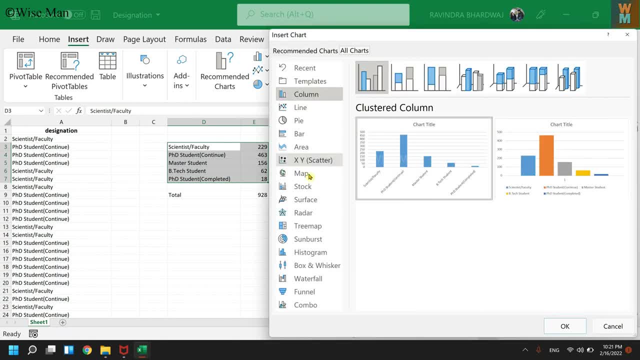 do click on all charts and from this you can uh select an appropriate chart which you want. over here. i want to be, i want to use pie chart because it is, because it is satisfying my conditions and it is, uh, it will look fine for me and then i will select the chart i. 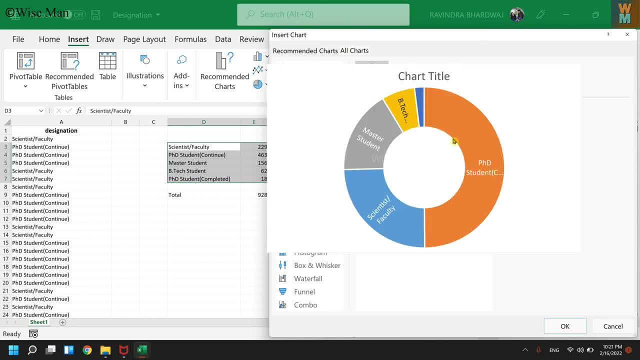 want for this if i was sunburst. you can see that it is not giving me the amount, the values, you can do that, but pie chart is a common one which is very useful. so we will use this pie chart, and over here there are different types of pie charts, so we have pi 3d, pi pi. 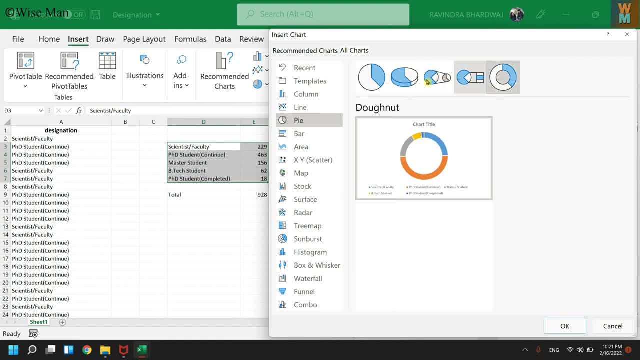 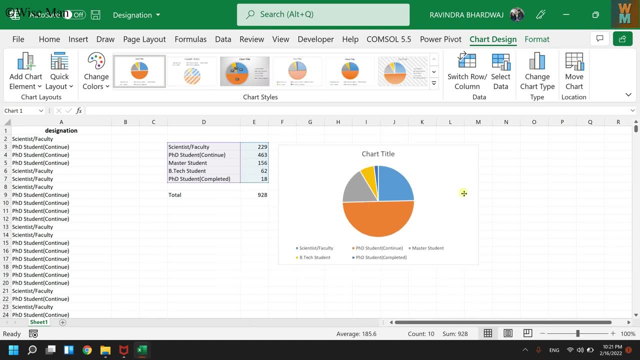 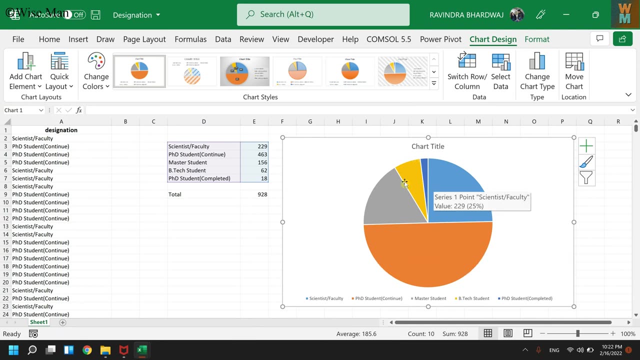 of pi, bar of pi and donut right. so let's use this one. click on ok and that will give me a pie chart of this values. right now you can see that uh, the values are not written over here. so for that, click on this right, click on that and click on uh for my data series, and then you can. 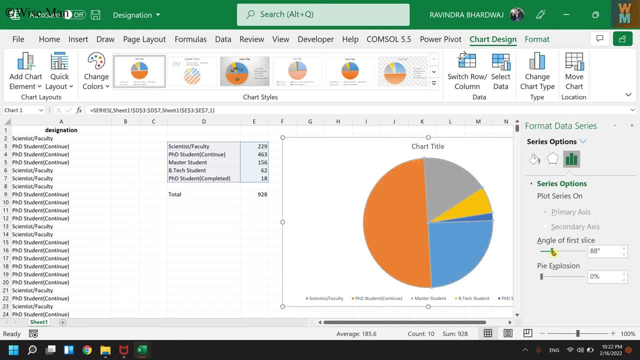 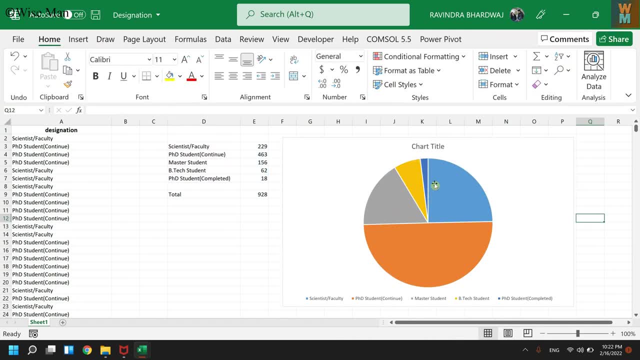 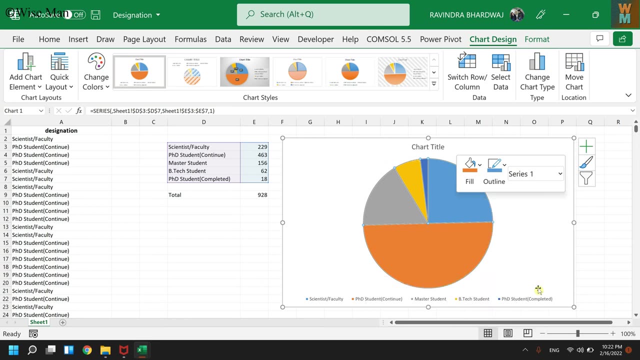 find some way that you can change this angle of slice, right? okay, so now to provide the values, to provide the actual values over here: right click on this, right click on that and provide: add data labels. right click on that and that will give you the data labels as: 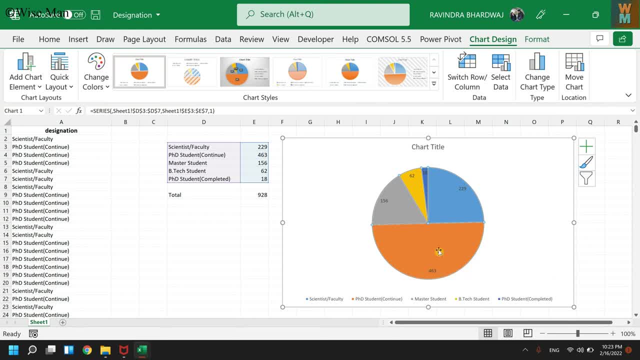 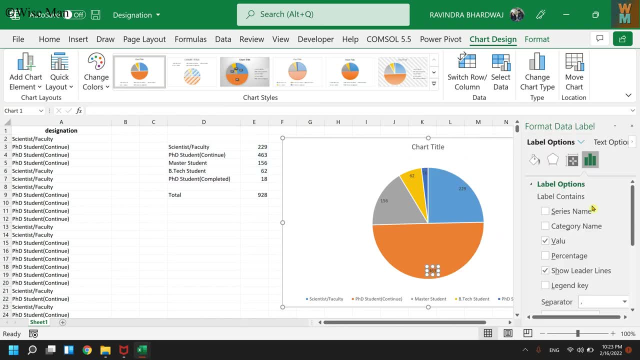 you can see over here right, so it will provide me the values over here. if you want um format, go to format data label and if you want percentage, click on that and that will give you simultaneously a percentage. if you want percentage of all, so click on this um, click on this whole chart. 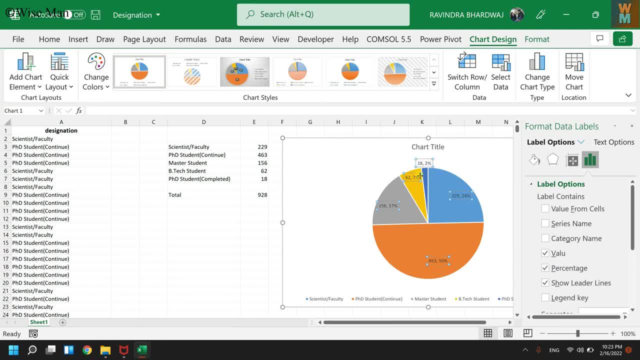 click on format data label and click on percentage, so that will give percentage. if you want only percentage, uncheck this and that will give you percentage over here. now this is the legend key. it has not required over here a category name you can select if you want to show that. 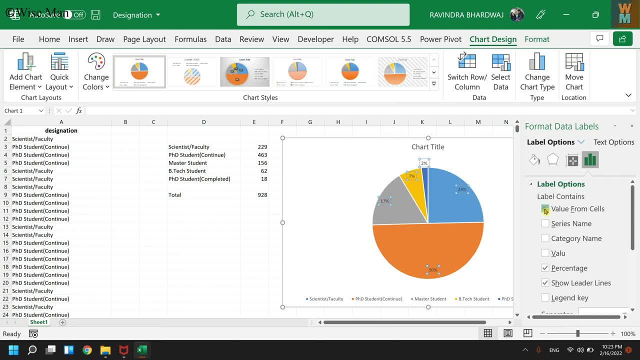 on the chart a series name, if you want, and value from cell, but it's not required for over here. right separator: you can select if you want to provide, like both the value and percentage. so that's um pretty much for this. from this you can position the uh, this um. 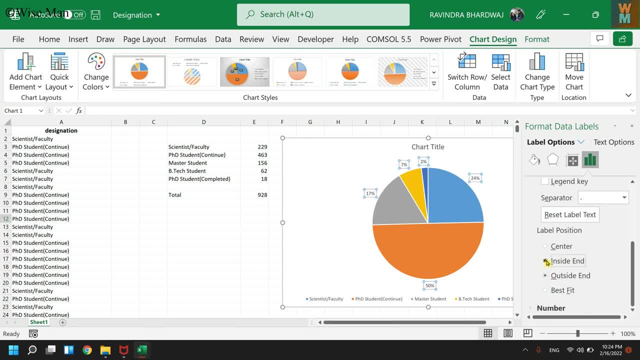 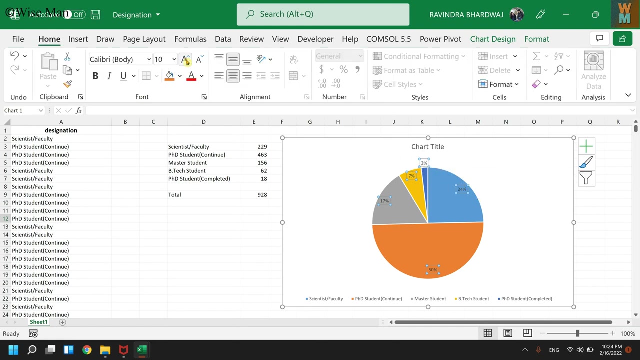 values right, best fit, uh, in outside, inside and or center best fit is generally, is usable, it will give. it will automatically uh. arrange these values as which is best fitted for the graph. now you can just increase or decrease the size of this font, so you the values are already selected. you can see that if you increase the font size. 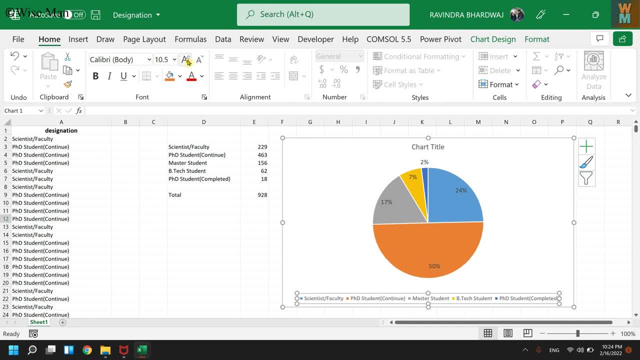 it will increase. select this legend, click on this. you can increase that. you can provide a chart title, so it is um, um. designation of participants. you can write whatever you, uh, you want to write, but for this it is the distribution of participants and you can just increase or decrease the font size of this. 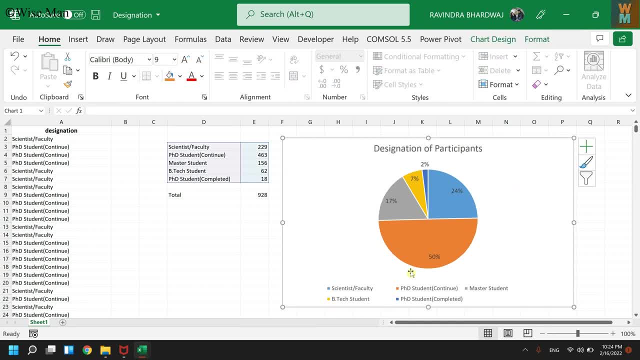 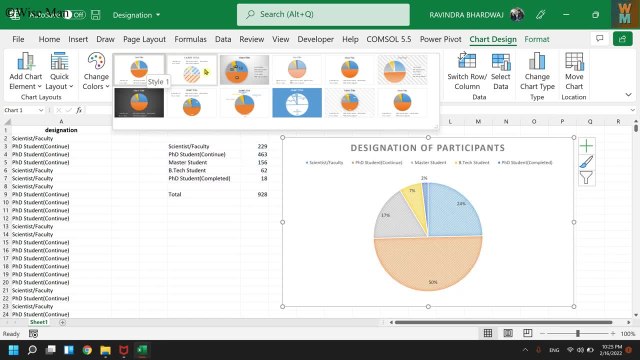 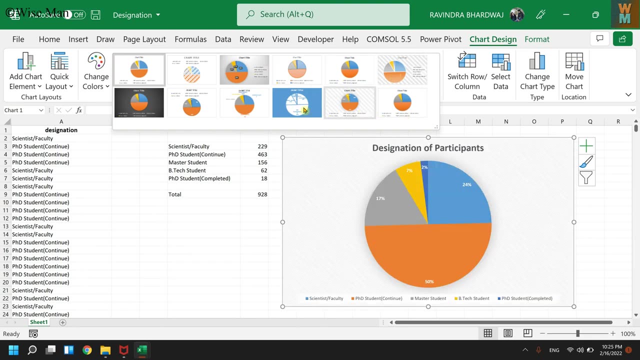 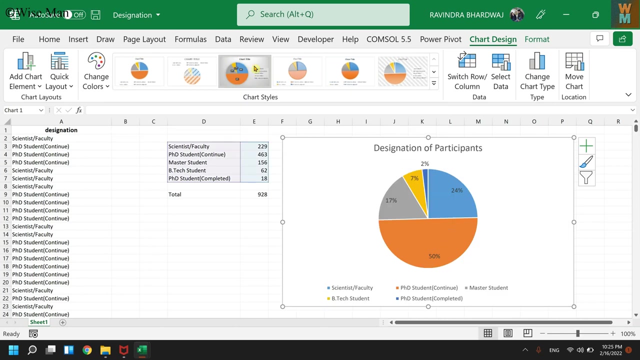 and you can change the background of this graph. go to chart design and you can see over here there are so many different types of styles that you can use. so, as you are seeing, it is various variety of. I am liking this chart so I will click on this. 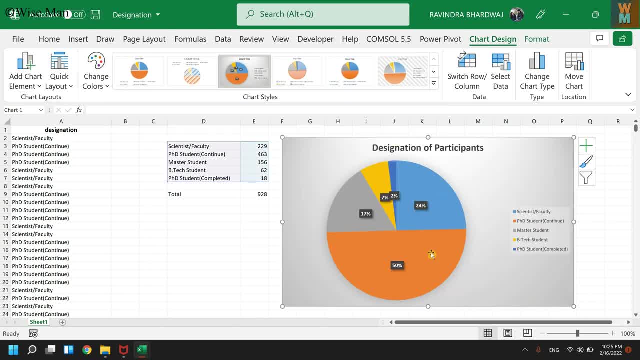 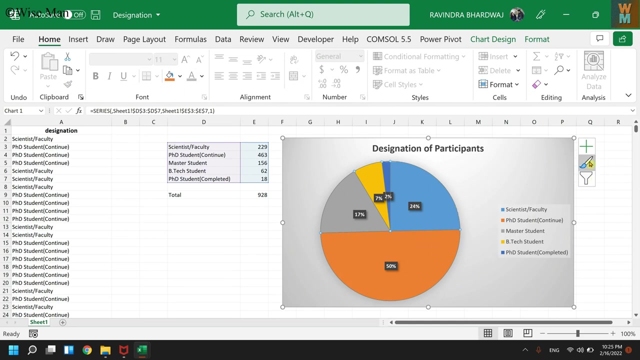 this design is looking very good for me and I can just play with this little bit to make it look good and increase the size if you want. okay, and then you can format it if you want, from here, from this side also. this is if you want to unselect or deselect something. 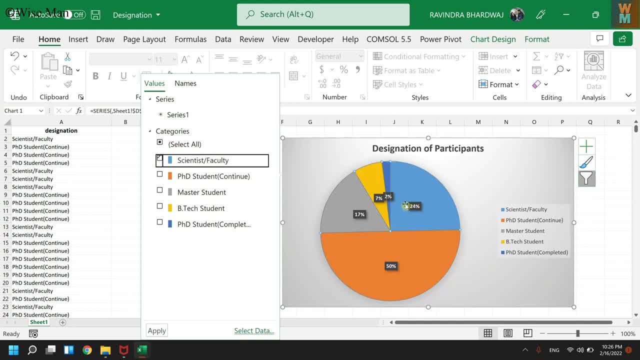 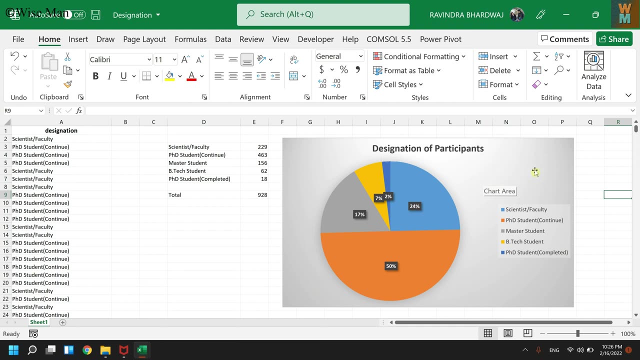 so that will give you. let's say, you just want to show this scientist faculty, it will show you that one. so that's up to you, okay, and then you can save this, save this image or save this graph. so right click on that right click and then click on save as picture. 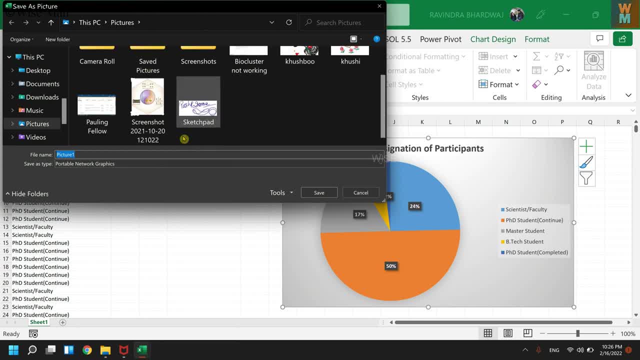 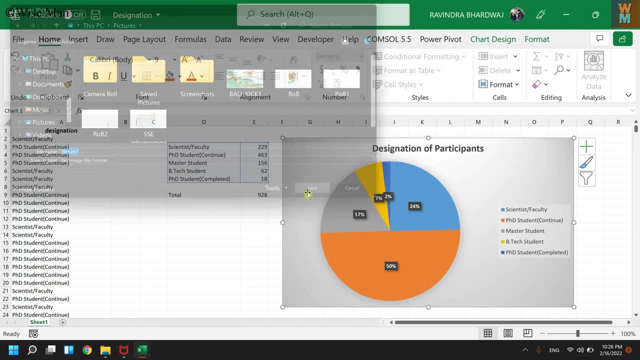 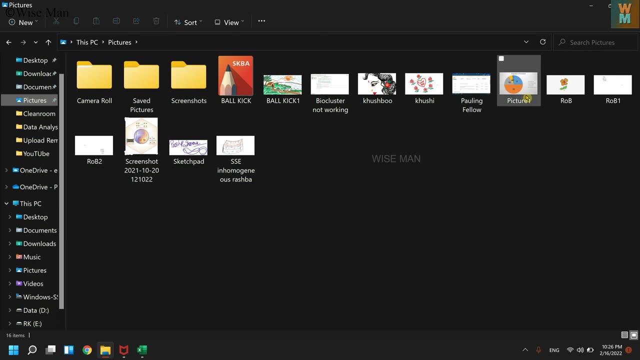 and then you can just save it over here, right, so you can select TIF format, which is very good, it's picture. one click on save and then you can go to documents, or I think it's pictures, and then it's over here. so it's 645 KB picture and if you open that 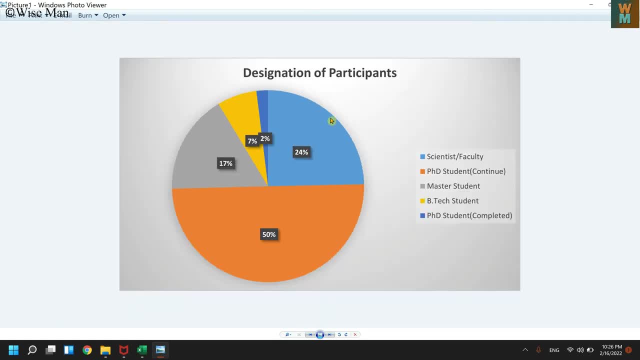 you can get the picture of this graph, so that way you can generalize the data, you can differentiate the data, you can just quantify the data and then you can make a chart from that. and that's all for this video. if it help you like, hit the like button.